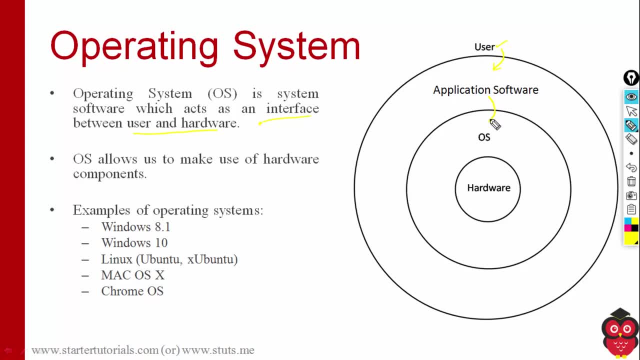 and this application software will pass requests to operating system and then operating system will interact with hardware devices like keyboard, mouse, monitor etc. So in general a user never interacts with hardware devices directly. they always interact with the computer using application software or in special cases. 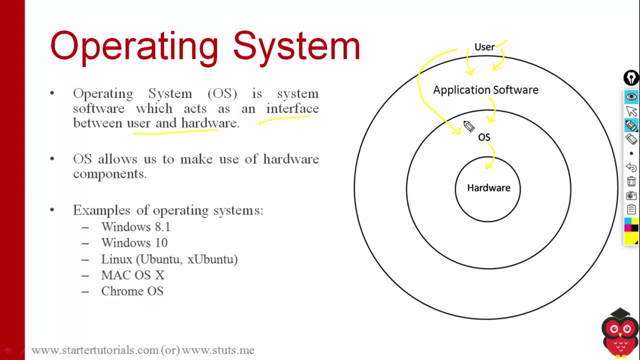 they will directly interact with operating system using some special software. and what is the use of operating system means? operating system allows us, the user, to make use of hardware component. so to use hardware there must be software, and one category of software is system software and where the operating system is an example for this term, software. so operating system provides code which 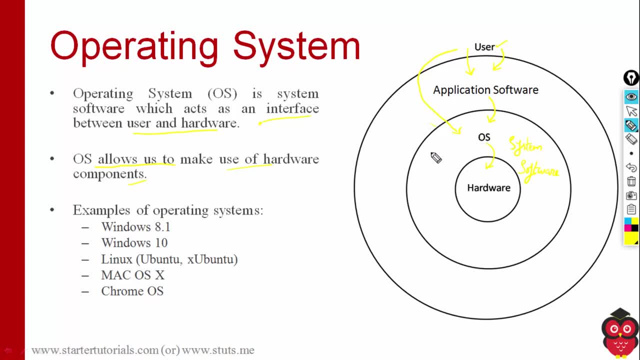 is common to all the application software like it for word over access keyboard, over the access to all the application software like it provide, or to access keyboard, or to access system, so in the monitor, so on and so forth. and some popular examples of operating systems used in desktop, computer, laptop or Windows 8.1 and latest version is Windows. 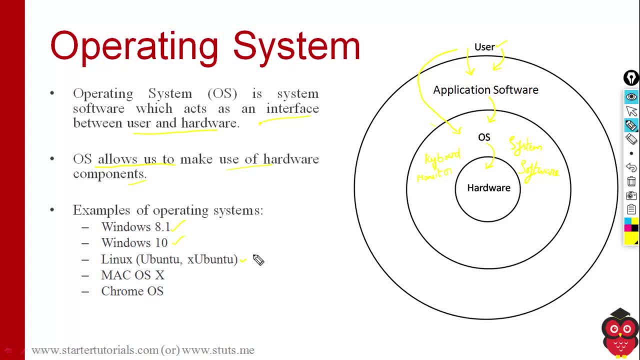 10, and we have open source operating system like Linux, and we have an operating system which is developed by Apple organization- the OS is Mac OS 10- and we have an operating system which is developed by Google and operating system name is Chrome OS. and we have also mobile devices. mobile devices use. 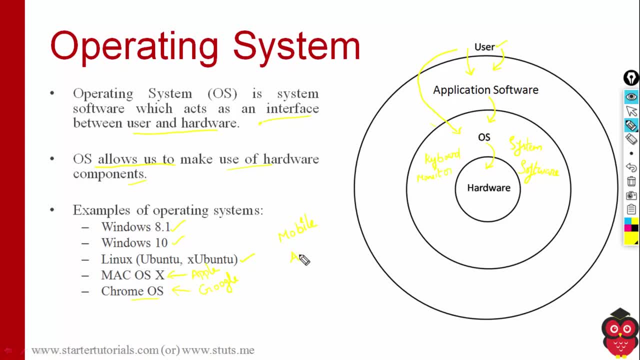 operating systems like Android, and if you have blackberry phone, they use blackberry OS. in some world, phones use mbion OS, so, and Windows phones use Windows mobile OS. so these are all examples of operating systems used in mobile. so now let's look at memory hierarchy. so there are various memory components in a 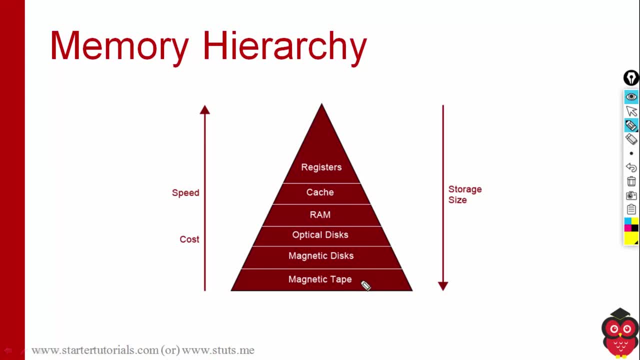 computer. there are magnetic tapes like which look like tape cassettes, which contains a magnetic tape where you store data. generally, magnetic tapes are used for taking backups and there are. There are hard disk devices, also called magnetic disk, and we have optical disk, which are CDs. 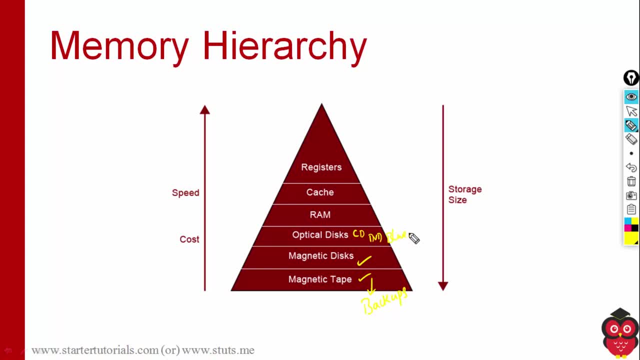 DVDs, Blu-ray disks- all these are optical devices And we have the primary memory, RAM, and we have another kind of memory called cache memory. So the use of cache memory is whenever there is some code in the RAM which is accessed frequently. that means it is being executed again and again and again such kind of code. 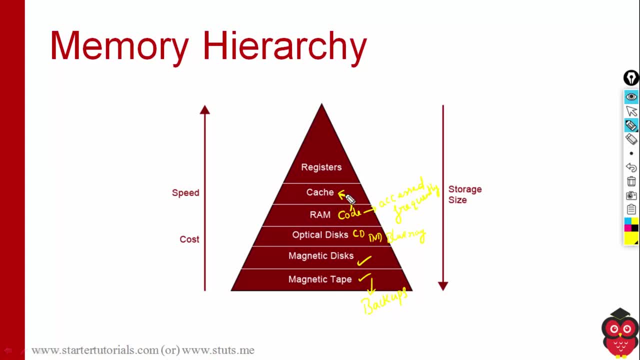 is loaded into cache memory. Why? because cache memory is faster than RAM, So CPU spends less time with cache than with RAM And these registers which are located within CPU. these are very faster devices when compared to rest of the memory components. So you can see various factors here in the hierarchy. 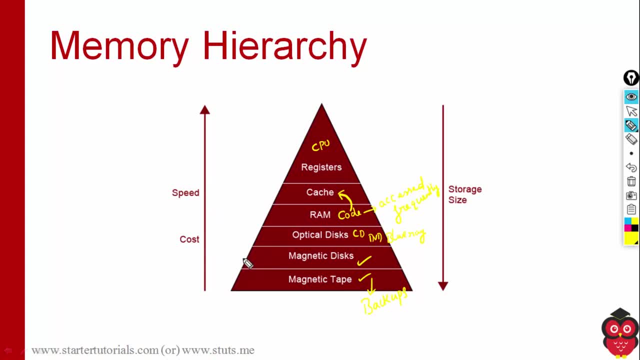 So if you take cost of this memory component, cost increases from top to bottom and also speed increases from bottom to top, Whereas storage size decreases from top to bottom. If you consider resistors and magnetic tapes, resistors are very small in size but they